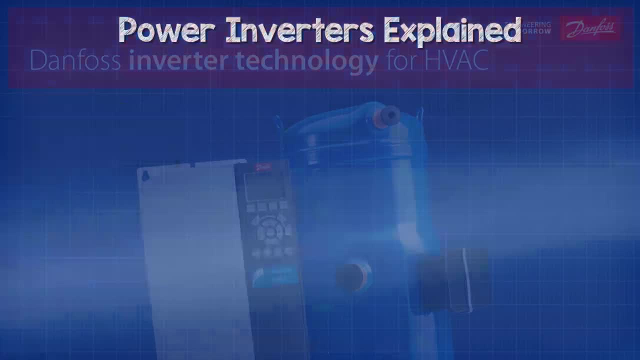 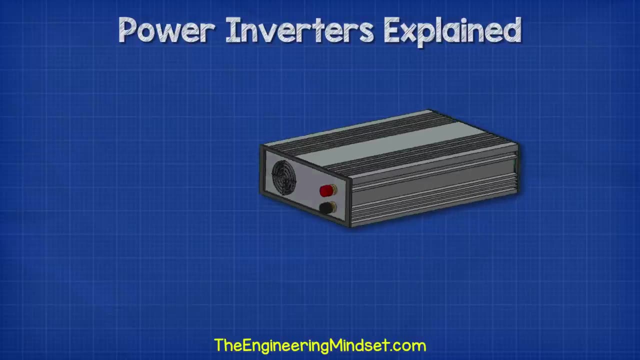 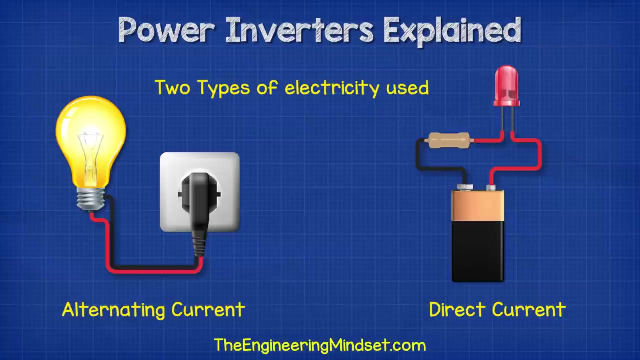 out any electrical work. A typical inverter looks something like this. It has some red and black DC terminals on the back end and on the front end we find some AC electrical outlets. That's because there are two types of electricity: there is AC and there is DC. An inverter is used. 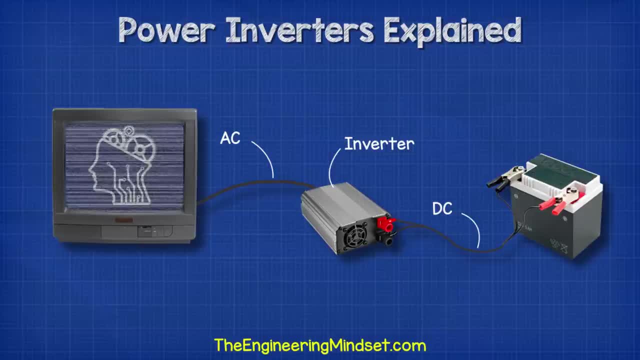 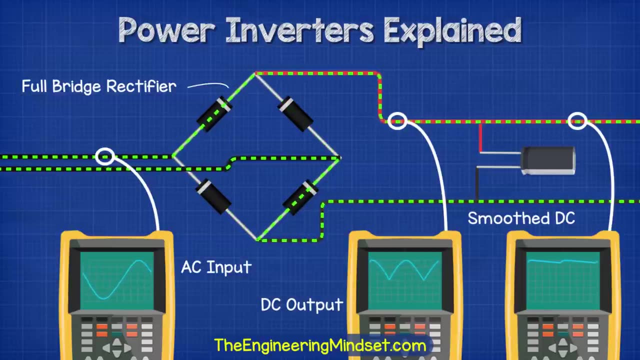 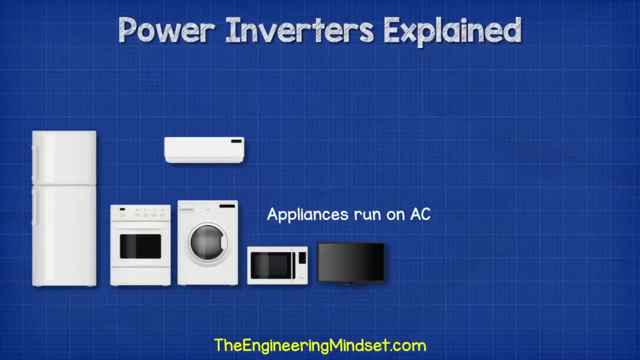 to convert DC or direct current into AC: alternating current. We can also convert AC into DC with the use of a rectifier, but we'll cover that in a separate video and I'll leave some links in the video description down below for that. The appliances in our homes are designed to run off of an AC supply and they get that. 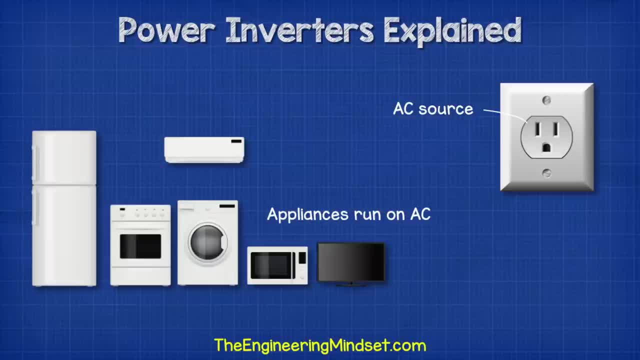 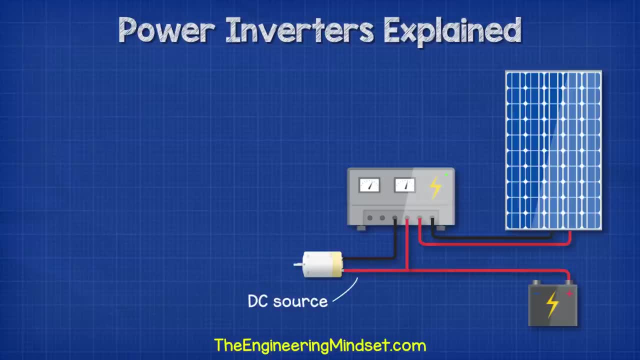 from the electrical outlets, which all provide AC electricity. However, electricity produced by things such as solar panels and batteries produce DC electricity. So if we want to power our electrical devices from renewable sources, battery banks or even our car, then we need to convert DC electricity into AC electricity, and we do that with an inverter. 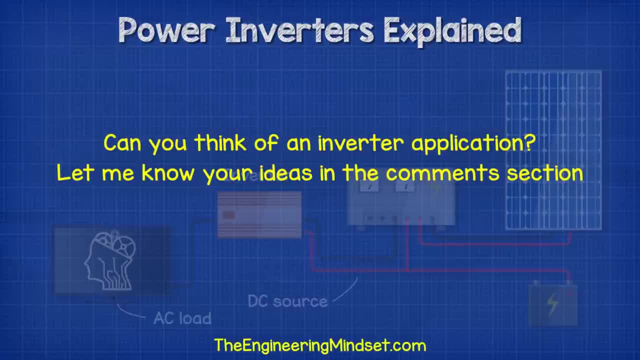 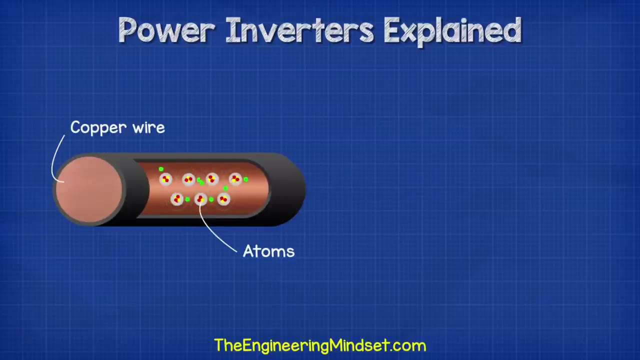 Where have you seen inverters used or where would you like to use one? Let me know your thoughts and your project ideas in the comments section down below. To understand how an inverter works, we first need to understand some fundamentals of electricity. Inside a copper wire we find copper atoms. These have electrons which can move to other 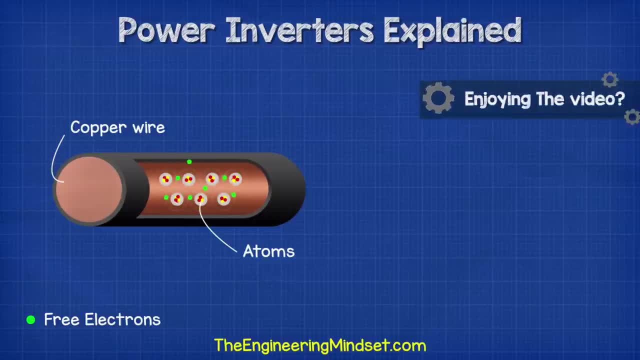 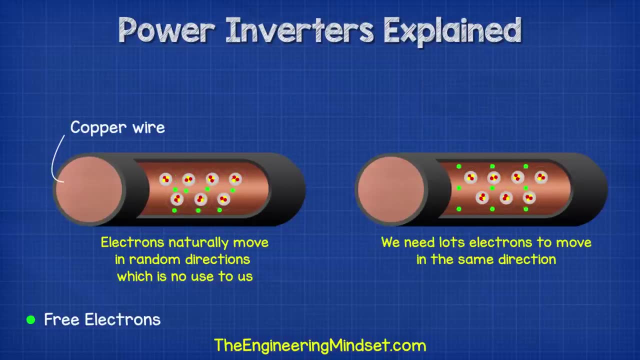 atoms. These are known as free electrons because they are free to move around. They will randomly move in all directions, but this isn't of any use to us. We need lots of electrons to move in the same direction, and we do that by applying a voltage difference across the 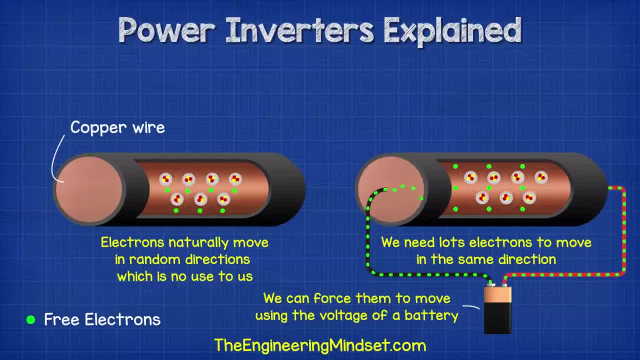 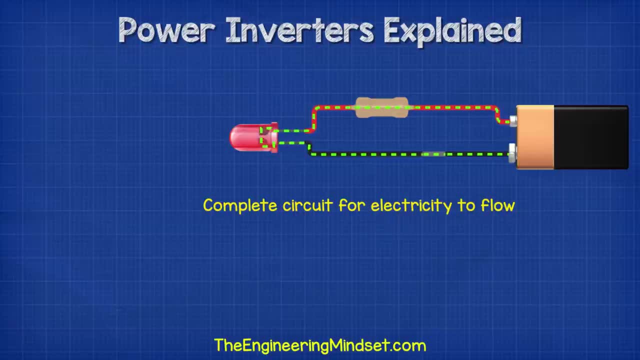 wire. The voltage is like pressure and will push the electrons. When we connect a wire to the positive and negative terminals of a battery, we complete this circuit and electrons begin to flow. We call this flow of electrons current. The electrons always try to get back to their 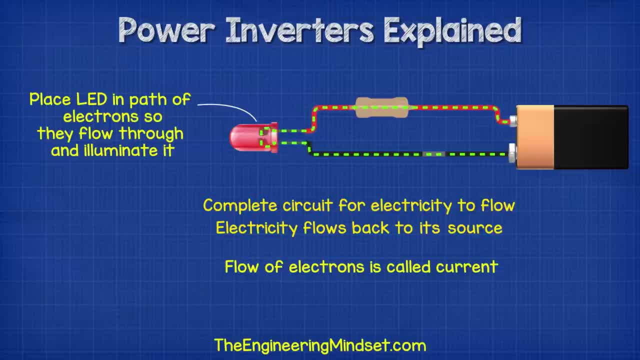 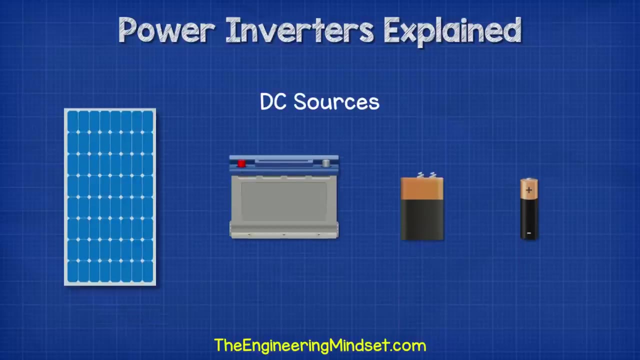 source. So if we place things such as lamps in the path of the electrons, they will have to pass through this and they will therefore do work for us, such as illumining this lamp. Electricity from an electric адjustment lamp, solar panels and batteries is known as DC electricity, and that's because this type of 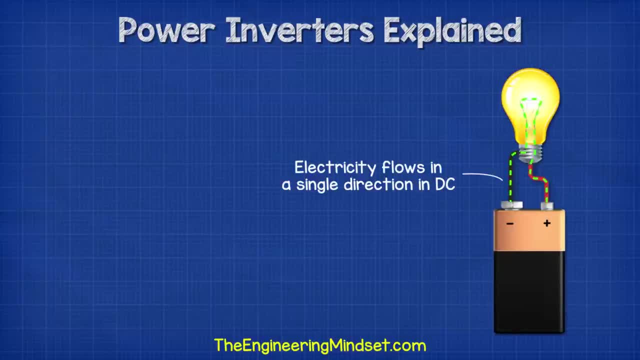 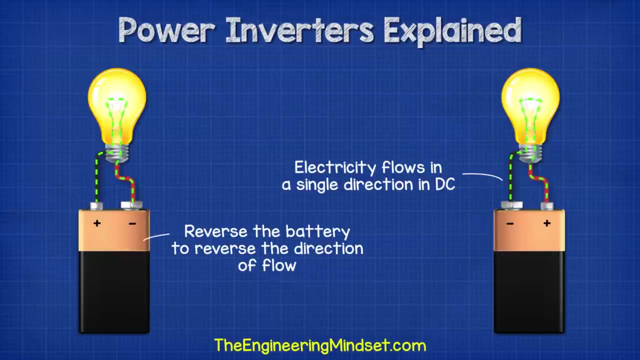 electricity flows in just one single direction. It flows from one terminal directly to the other terminal. If we reverse the battery, the electrons flow in the opposite direction. You can think of DC electricity like a river, with the current of water flowing in just a single direction. 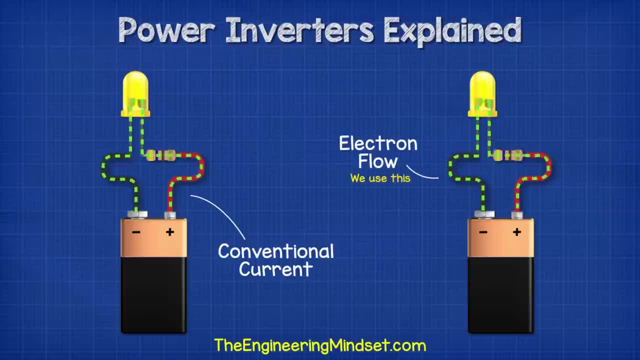 Now, in these animations I use electron flow, which is from negative to positive, but you might be used to seeing conventional current, which is from positive to negative. Electron flow is what's actually occurring. Conventional current was the original theory and it's still widely taught today. 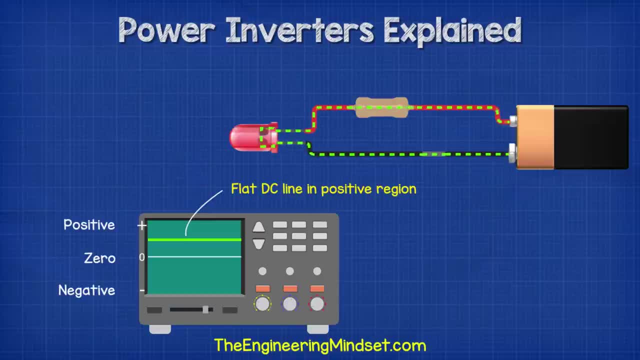 Just be aware of the two and which one we're using. When we use an oscilloscope to look at the electrical waveform for DC, we get this flat line at the maximum voltage in the positive region. If we were to cut the power then the line will drop to zero. If we turn the power on and off, 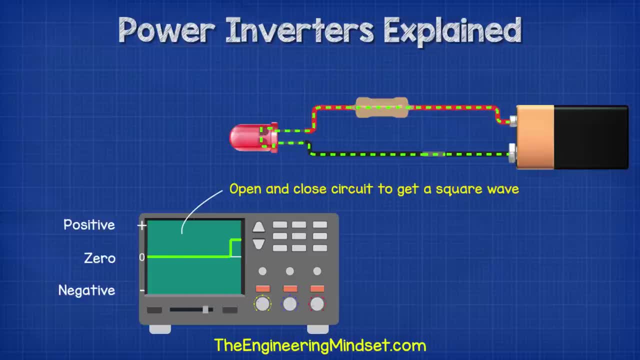 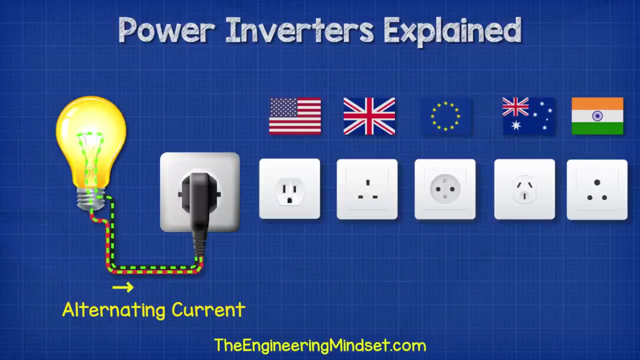 repeatedly, then we get a square wave pattern Between zero and maximum. But if we were to pulse the switch to open and close over different lengths of time, then we would get a pulsating pattern. With AC electricity the electrons alternate by flowing forwards and backwards constantly. That's how it gets its name, because the current of 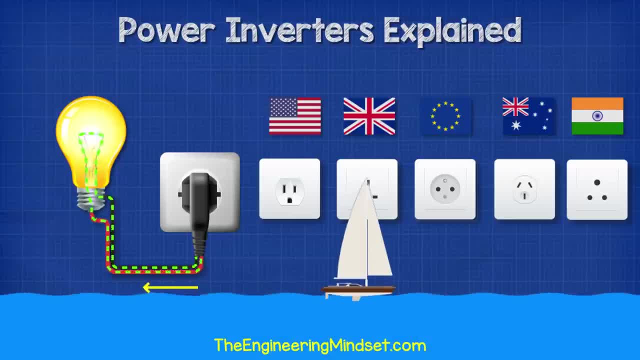 electrons alternates in direction. You can think of this type of electricity like the tide of the sea. It constantly flows in and out between the maximums of high tide and low tide. If we followed the copper wires back to the generator, the wires are connected. 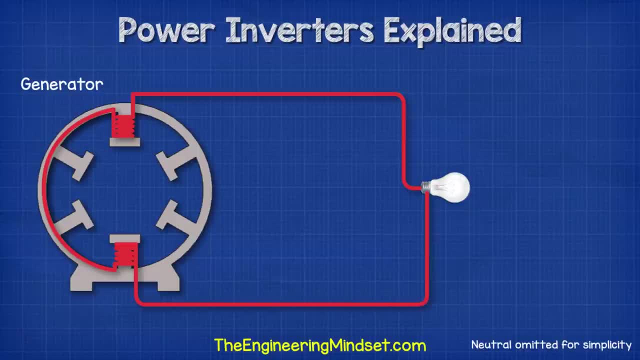 to some coils of wire which sit within the generator. Inside a basic generator, we also find a magnet at the center which is rotating. The magnet has a north and south pole, or you can think of it as a positive and a negative. half The electrons in the wire are negatively charged. 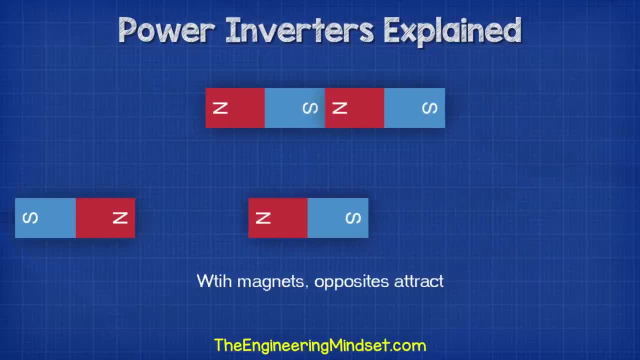 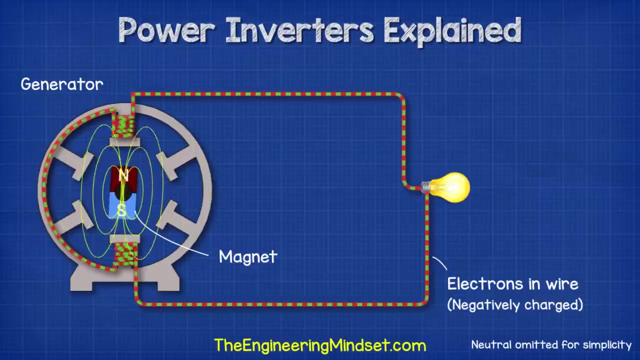 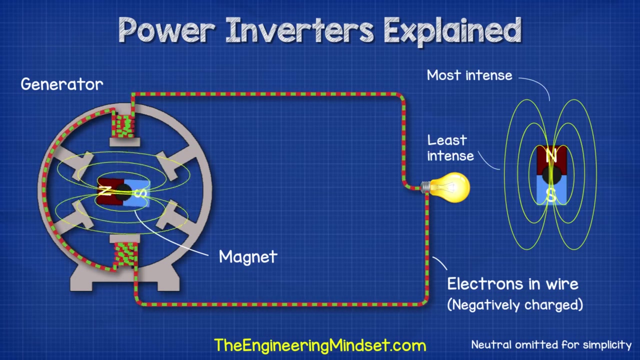 As you might already know, magnets push or pull depending on the polarity. So as the magnets rotate past the coils, the positive and the negative half are going to therefore push and pull the electrons within the copper coils and also through the connected copper wires. The magnetic field of the magnet varies in intensity, So as the magnet rotates past the coil. 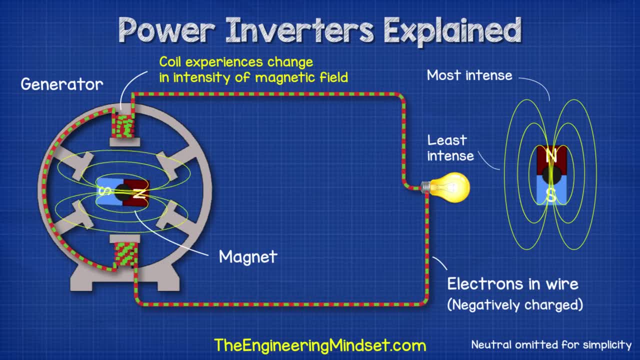 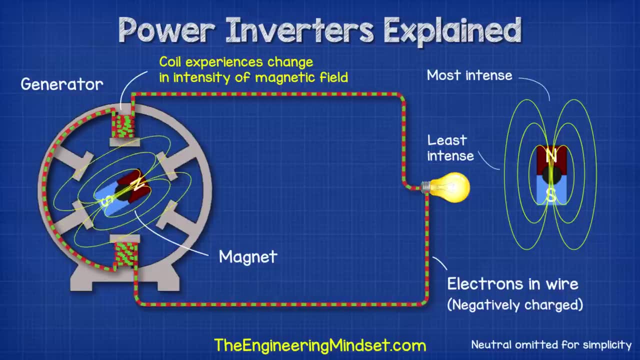 the coil will experience a change in intensity of the magnetic field. This will be from zero up to its maximum intensity and then, as it passes the coil, the magnetic field will change. It will decrease again back to zero. Then the negative half comes in and pulls the electrons. 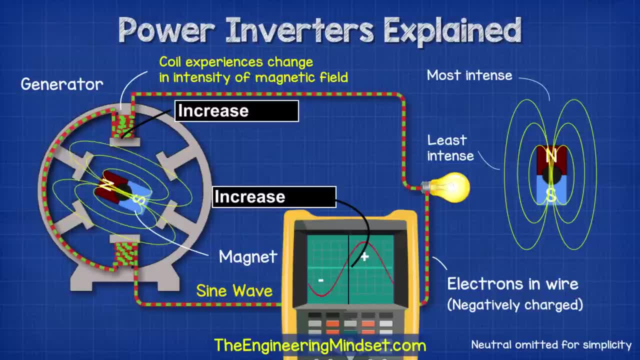 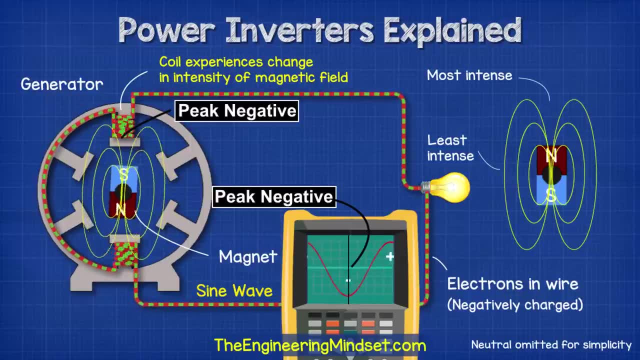 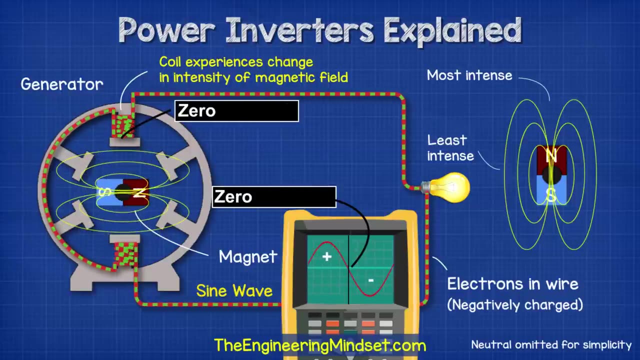 backwards with the same change in intensity. Each full rotation of the magnet will therefore produce this wave pattern, known as a sine wave. The voltage is not constant in this type of electricity. Instead, it repeatedly moves from zero up to its peak, back to zero, then to the 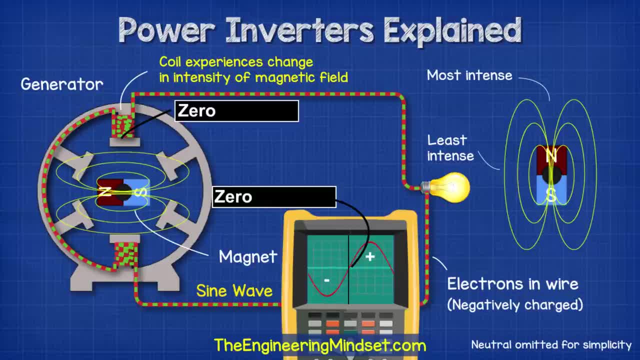 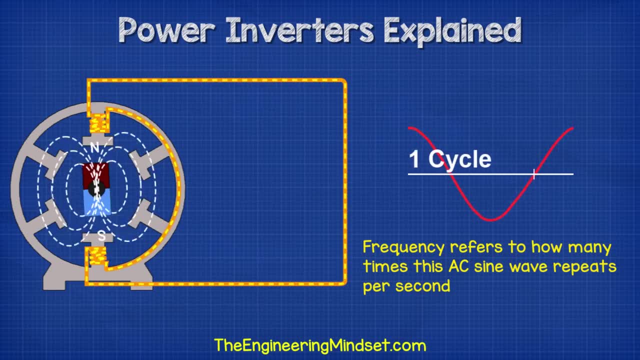 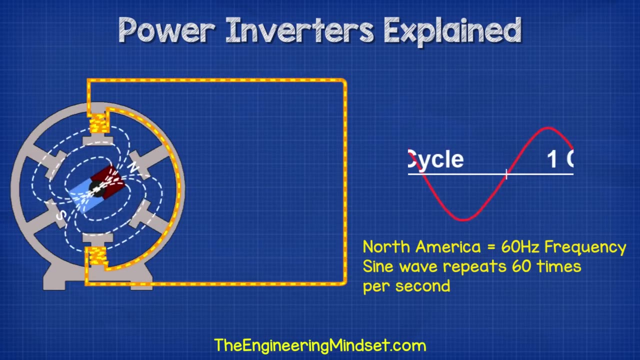 negative peak and then finally back to zero again. Frequency refers to how many times this AC sine wave repeats per second. In North America and a few other parts of the world we find 60 hertz electricity, which means the sine wave repeats 60 times per second And as each wave has a positive and a negative half, this means its 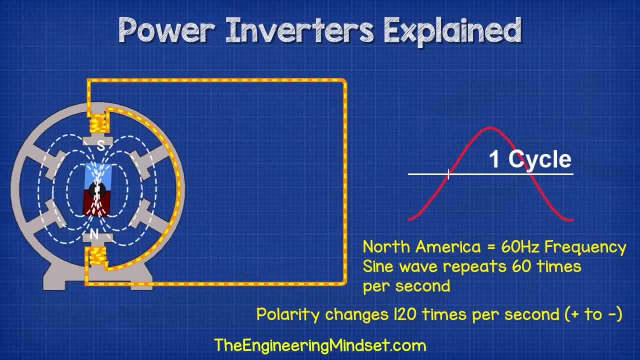 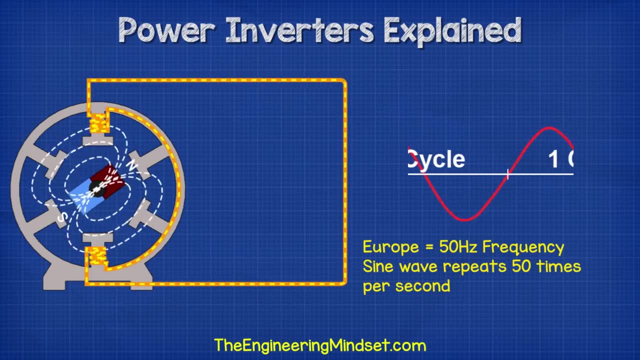 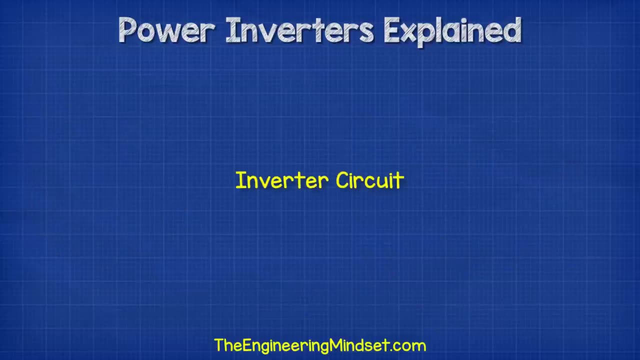 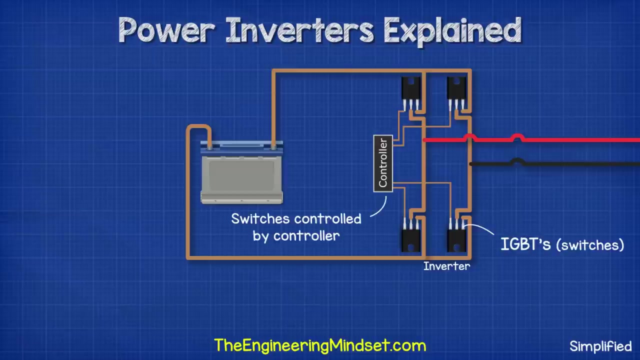 polarity will therefore reverse 120 times per second. In the rest of the world we mostly find 50 hertz electricity, So the sine wave repeats 50 times per second and therefore the current reverses 100 times per second. The inverter consists of a number of electronic switches known as IGBTs. The opening and closing. 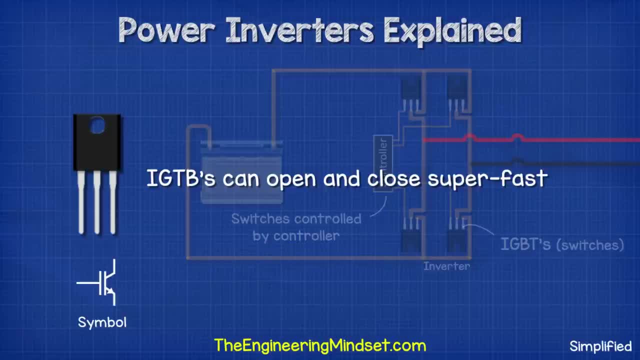 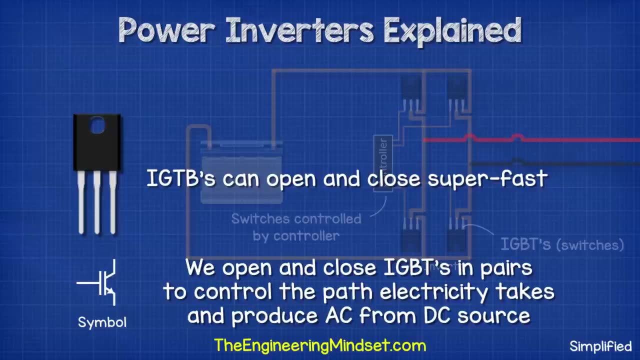 of the switches is controlled by a controller. These can open and close superfast in pairs to control the flow of electricity. By controlling the path which the electricity takes and how long it flows in the different paths, we can produce AC electricity from the DC. 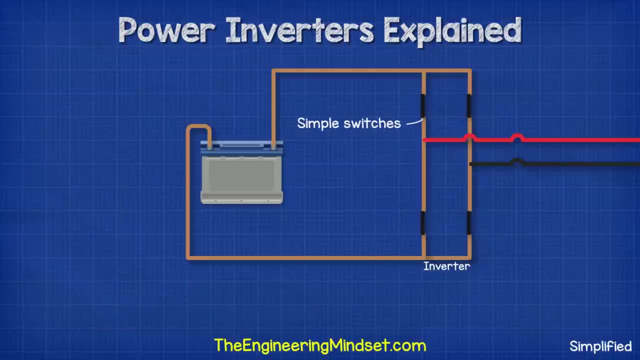 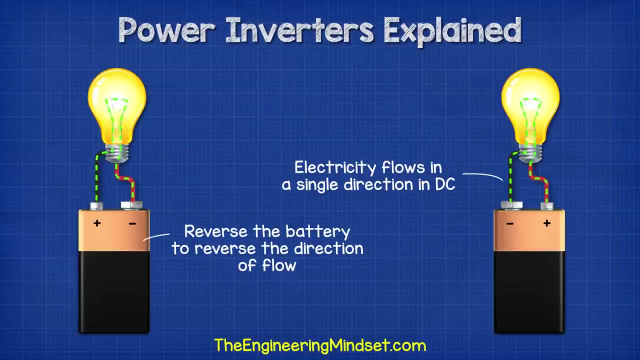 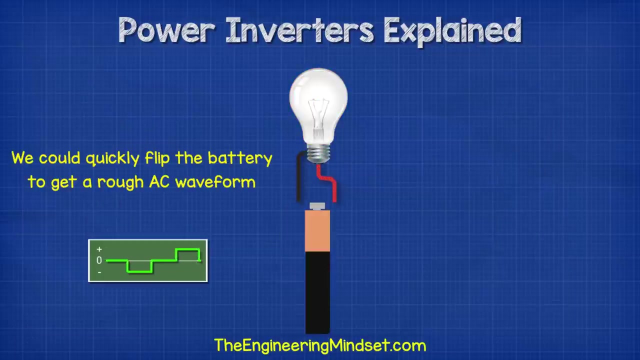 DC source. I'm going to animate these using some simple switches to make them easier to visualize. Remember, AC is where the current reverses direction. We saw earlier in the video we can reverse the direction of current by reversing the battery. We could very quickly reverse the battery to produce a rough AC. 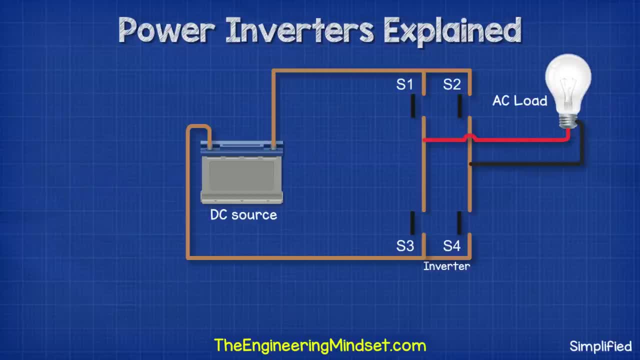 supply. but an easier way would be to connect four switches or IGBTs across our load such as a lamp. If we open and close these in pairs then we can produce AC electricity. So if we were to close switches one and four, then the current. 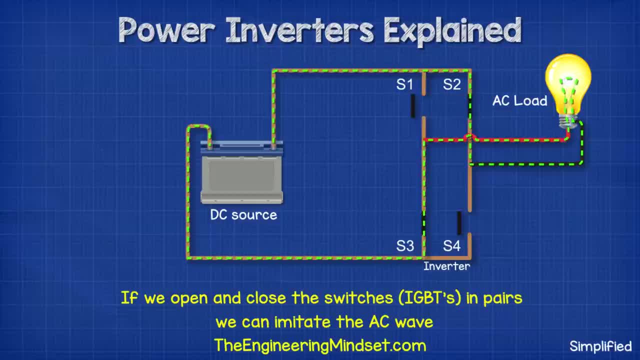 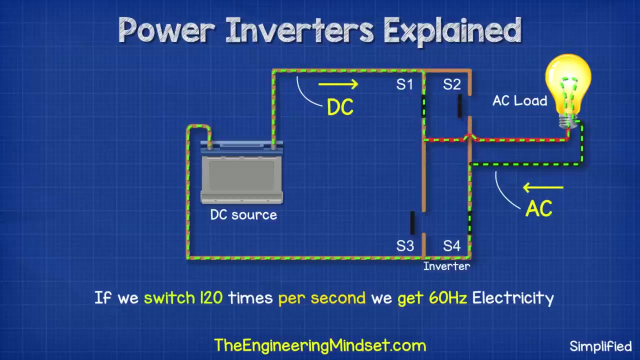 flows in one direction, and if we then open these and close switches two and three, we get current flowing in the other direction. So we can use the controller to automatically do this again, and again, and again. If we did that 120 times per second then we would get 60 Hertz electricity. 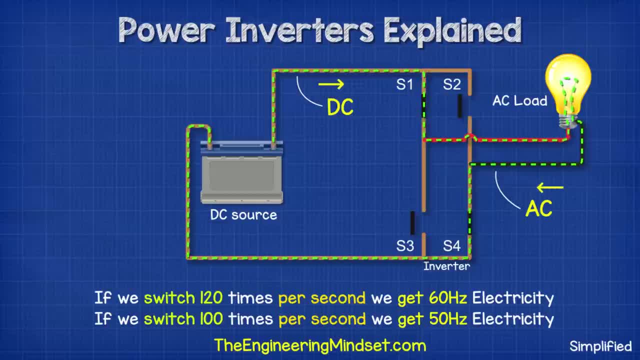 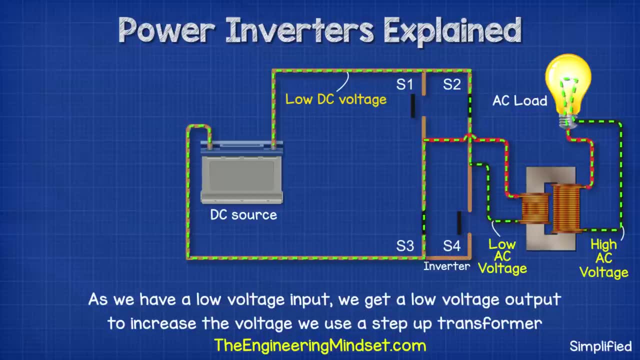 And if we did that 100 times per second then we would get 50 Hertz electricity. As we have a low voltage input, we're going to get a low voltage output To reach the 120 volts or 230 volts required to power our appliances. we will 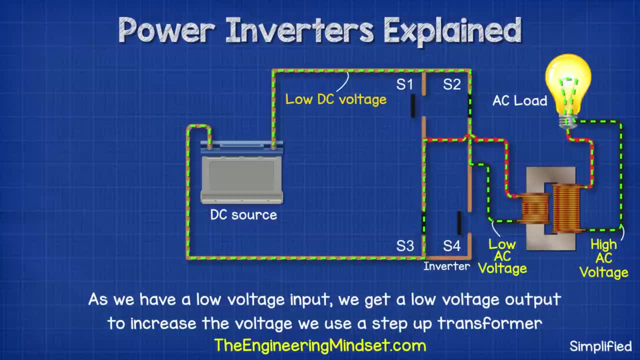 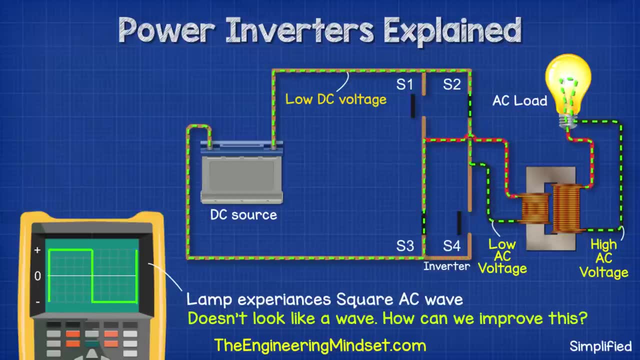 also need a transformer to step up the voltage to a useful level. When we look at this through an oscilloscope, we get a square wave in the positive and the negative regions. This is theoretically AC because it reverses direction, But it doesn't really look much like an AC sine wave. So how can we improve this? 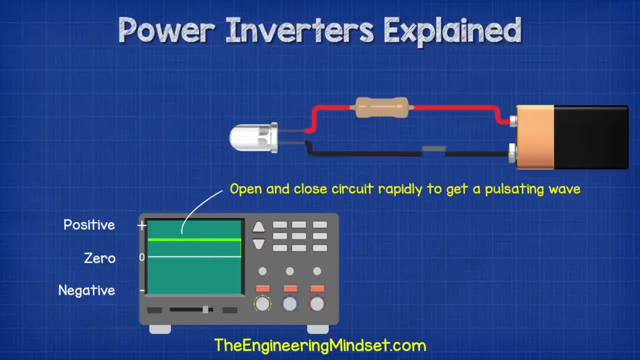 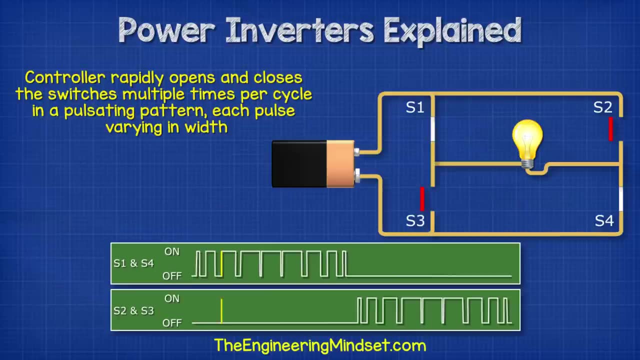 Do you remember earlier in the video when I said we can open and close the switch at different speeds and durations to change the waveform? Well, we can do that for this too. What we do is to use a controller to rapidly open and close the switches multiple times per cycle in a pulsating pattern, Each pulse varying in. 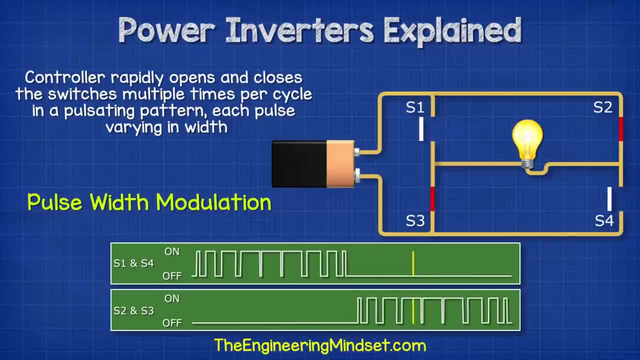 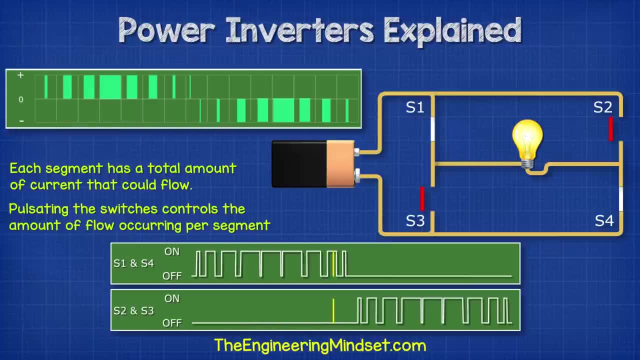 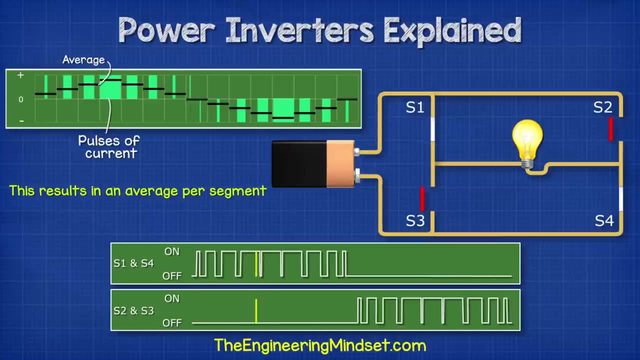 width. This is known as pulse width modulation. The cycle is broken up into multiple smaller segments. Each segment has a total amount of current that could flow, But by rapidly pulsating the switches we control the amount of flow occurring per segment. This will result in an average. 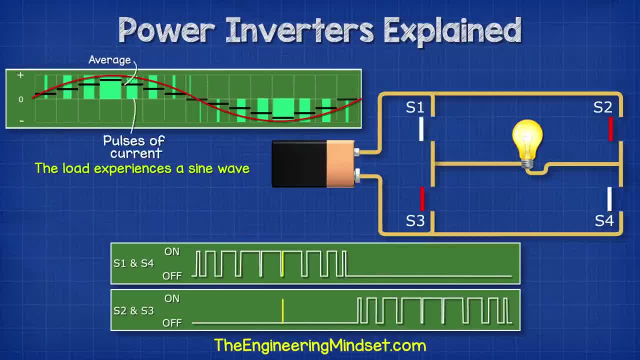 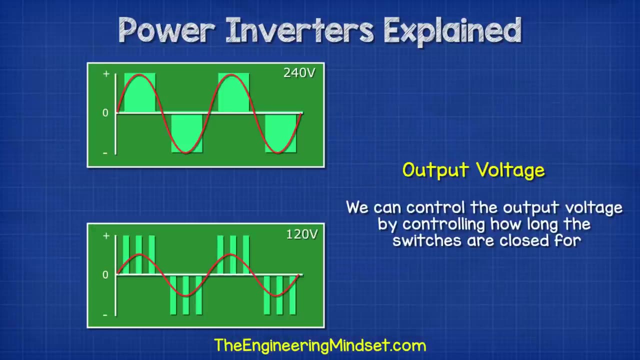 current per segment, which we see increases and decreases, thus giving us a wave. The load will therefore experience a sine wave. The more segments we have, then, the closer it mimics a smooth wave. We can control the output voltage by controlling how long the switches are closed for. So we could, for example, 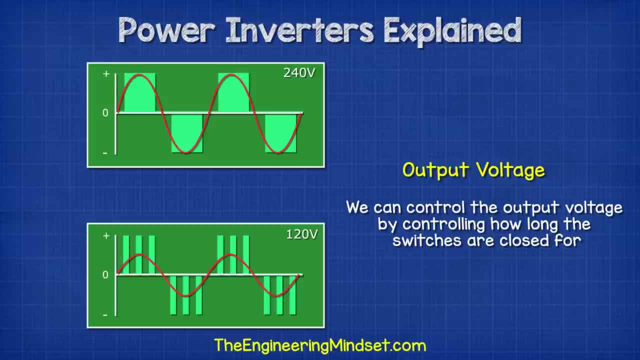 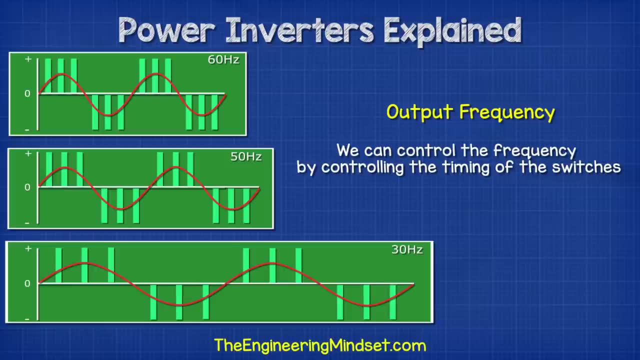 output 240 volts or 120 volts just by trimming the opening and closing times. We can also control the frequency by controlling the timing of the switches. So we could, for example, output 60 Hertz, 50 Hertz or 30 Hertz, whatever is needed. 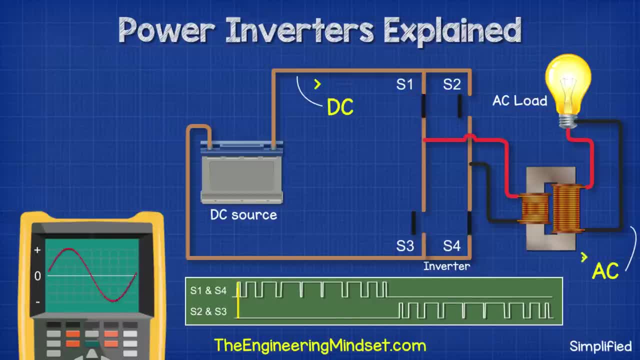 for the application. So that's how we can take a 12 volt DC battery and convert this into a 120 volts or 220 volts DC. The AC supply is a 230 volt AC supply by using some IGBTs: pulse width modulation. 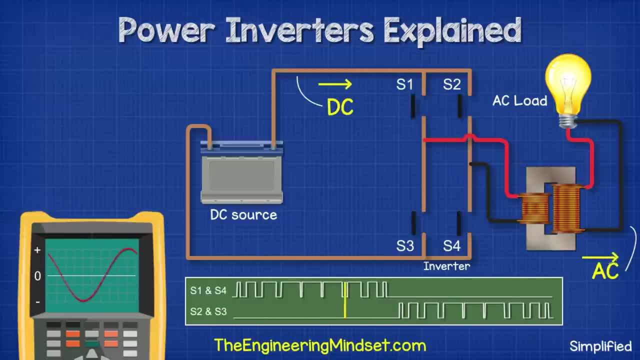 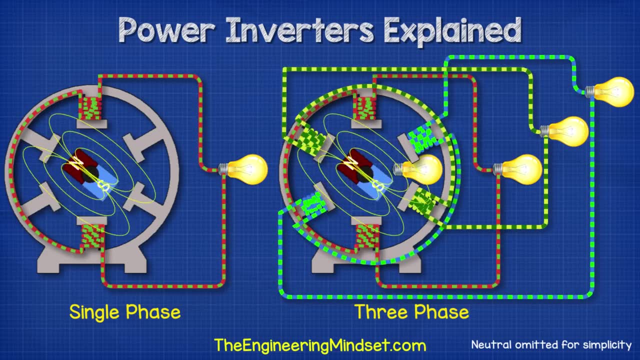 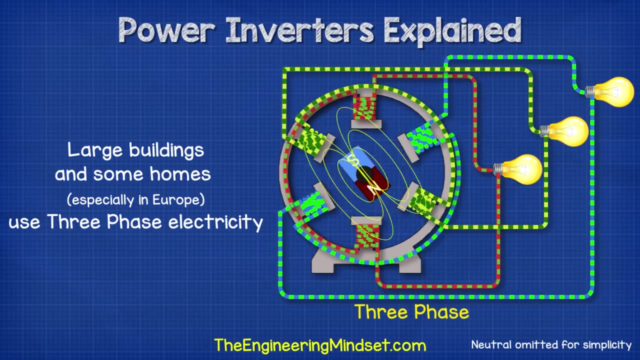 and a transformer. But what if we needed more power? We also have single phase as well as three phase AC electricity. Most homes around the world use single phase electricity. Large commercial buildings as well as some homes, especially in Europe, will use three phase electricity. Homes in North America use split. 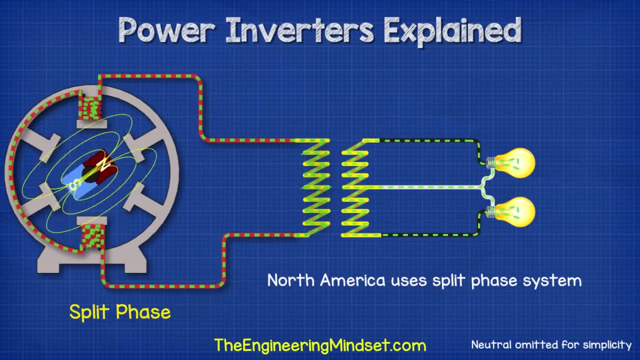 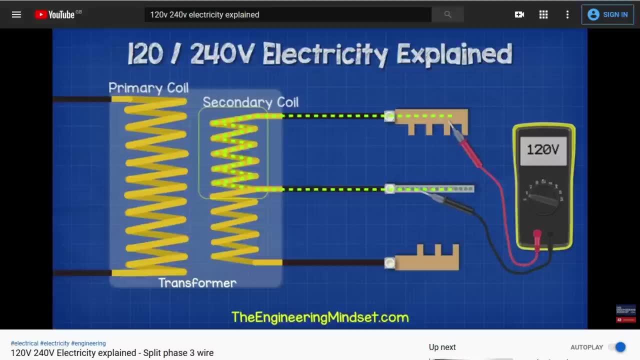 phase electricity Where a center tapped transformer splits a single phase into two, which provides two hot wires and a neutral. We've covered how split phase electricity works in detail in our previous video. Do check that out. links down below. With single phase we have a. 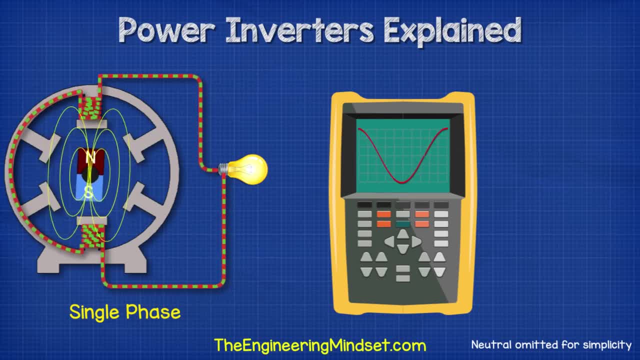 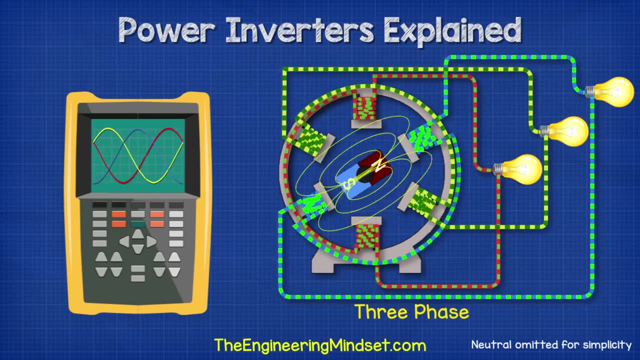 connection to just a single phase from a generator. So we have just one sine wave, But with three phase electricity we have a connection to each of the three phases. The phases are coils of wire which were inserted into the generator 120 degrees apart from the previous. 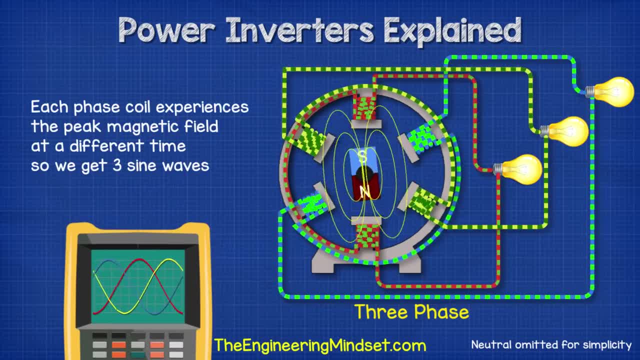 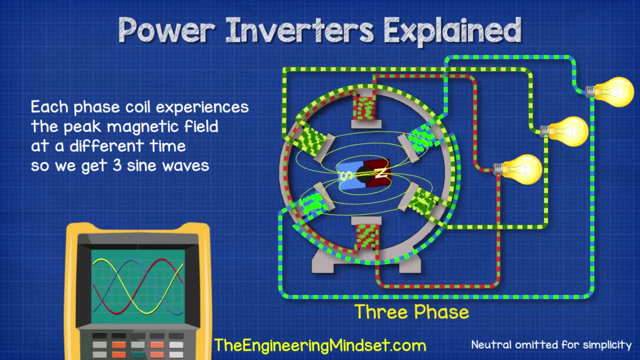 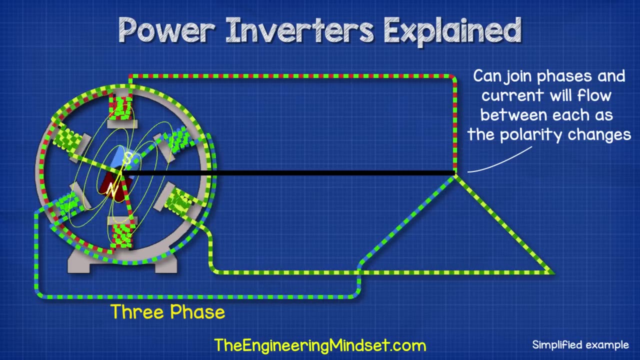 This means the coils experience the peak of the rotating magnetic field at different times, And it's this that gives us our three phases, Each with a different sine wave that is slightly out of sync from the previous. Remember, electricity wants to get back to its source in a complete circuit, As the current is flowing forwards and backwards at different. 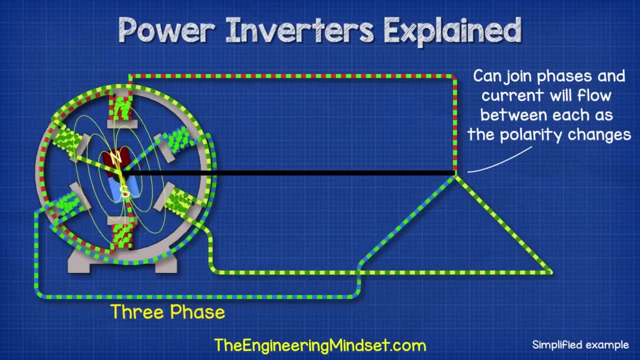 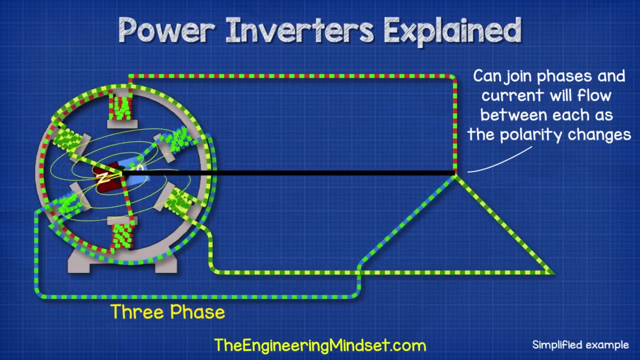 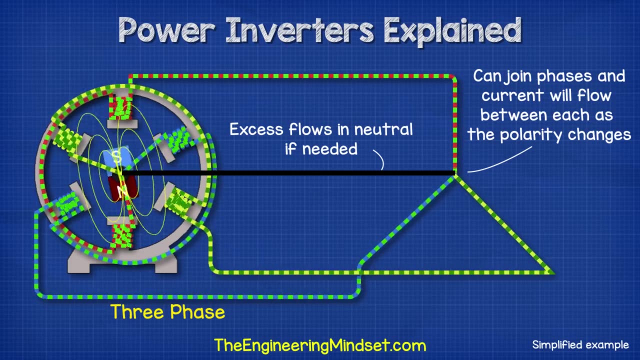 times in each of the phases. We can essentially connect the phases together and the current will move between the different phases as the polarity of each phase moves forwards and backwards at different times. Any excess will flow in the neutral back to the source if needed, But that's only if the load on any of the phases is unbalanced With single. 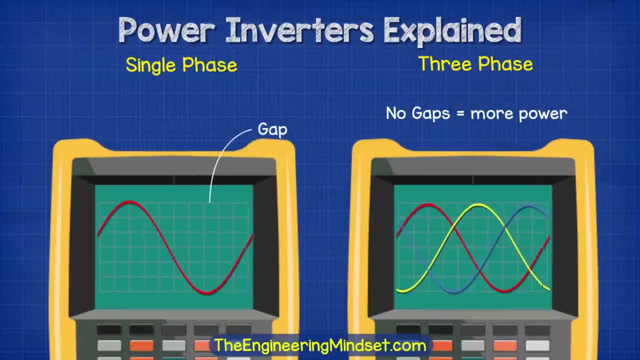 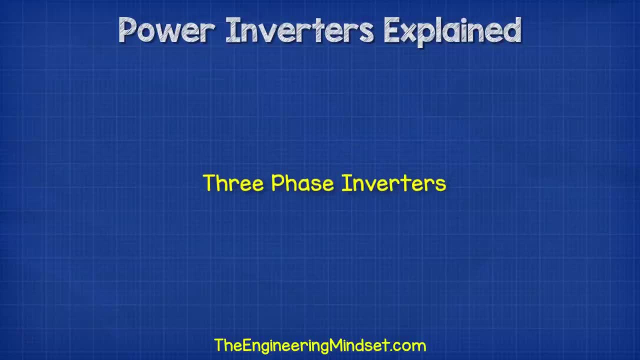 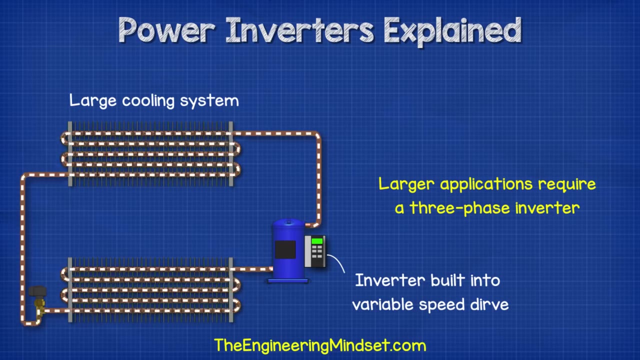 phase we have these large gaps between the peaks, But with three phase these can be combined to fill in the gaps and therefore deliver more power. Larger applications require a three phase inverter, For example to run the compressors in a large cooling system. The 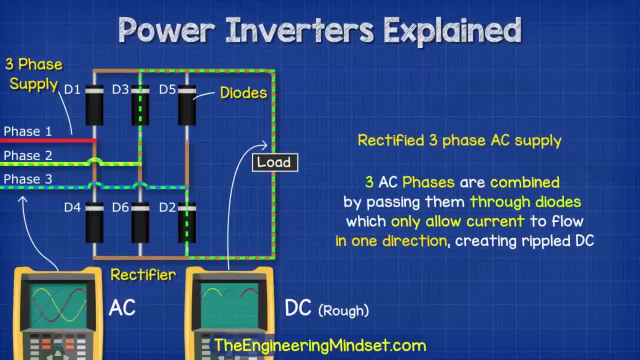 AC supply in this case will be a rectified three phase AC supply. That means the three AC sine waves are combined together and pass through some diodes which prevent the electrons from flowing backwards. This turns it into a ripple DC waveform. We then use a capacitor. 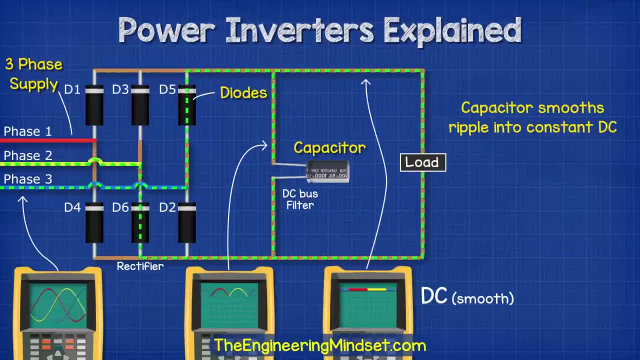 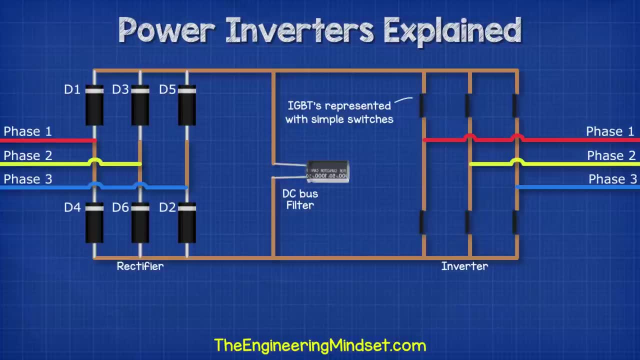 to smooth the ripple out into a constant DC supply. Now we have covered this in great detail previously. Do check that out the links down below. To turn the clean DC into a three phase AC, we use a three phase inverter. This means that the currentically flowing